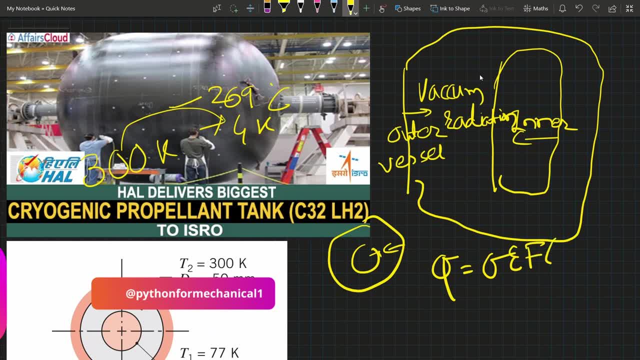 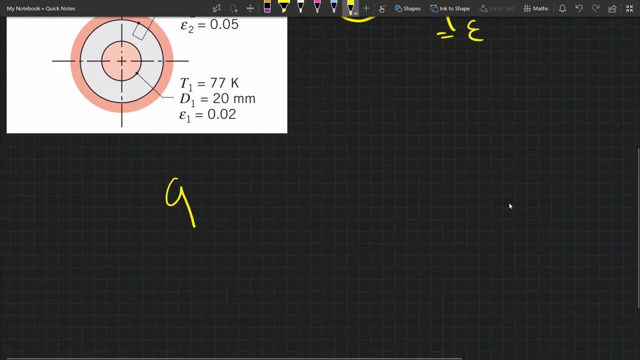 constant emissivity. our u factor and T raise to 4 minus T 2 raise to 4. so we know that our e is equal to our view. factor is equal to like this one. Q is equal to means different area: t 1 raise to 4, t 2 raise to 4 and 1 upon e 1. 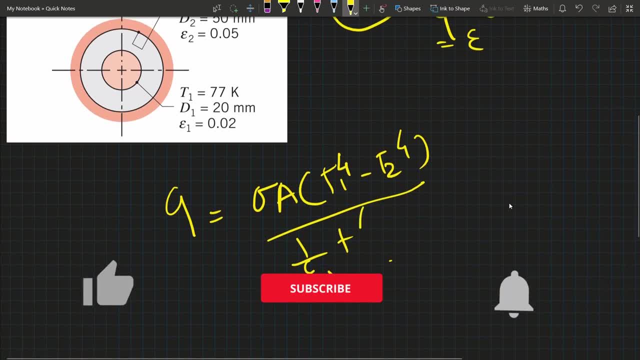 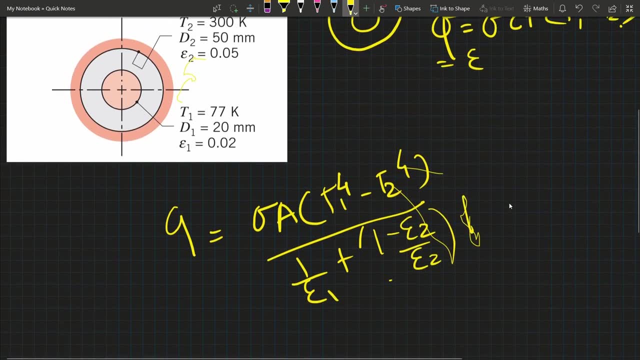 emissivity of this surface, plus 1, minus e 2, divided by e 2, emissivity of this surface and d 1 divided by d 2. this is the equation of our heat transfer of this cylinder. so now we will solve in this equation in Python and we will see what the effect. 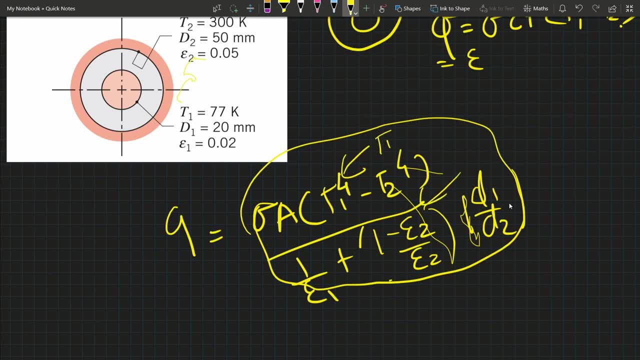 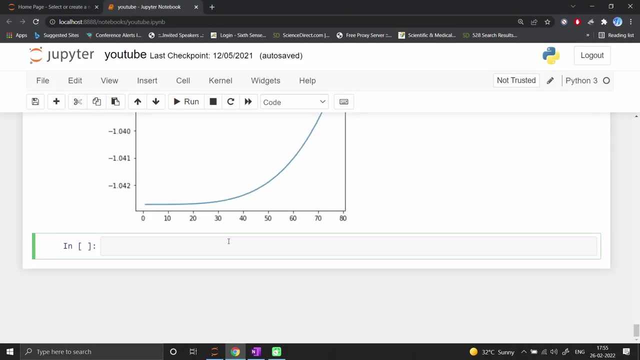 of this T 1 temperature and our emissivity. so now we'll go for it in Python. first we will import our numpy. numpy as NP, import matplotlib, dot py, plot as PLT and import math. now we'll see, Stefan Boltzmann, constant s is equal to five point six, seven. e raise to minus eight and our area means first we 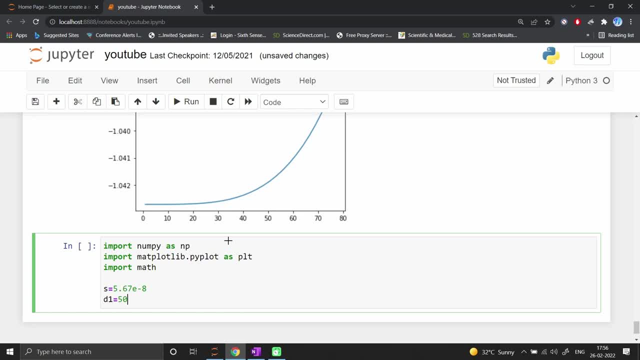 will define our diameter. d 1 is equal to 50 and we will divide into hundred the third one into��터. d2 is this: because of this, in Meter, D 2 is equal to around 300 divided by 1,000 in all meter, now, our area area is equal to a 1. 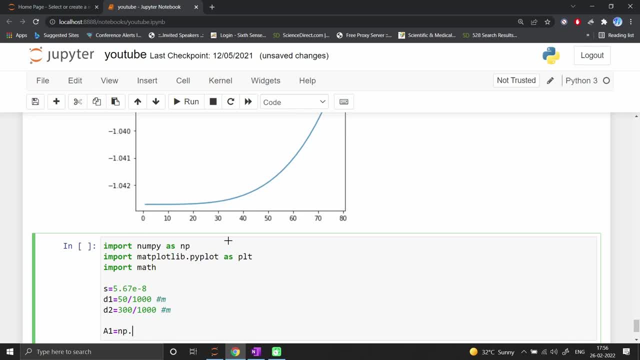 is equal to math. okay, I'll say num, NP, PI, multiply by 2 linhaMgetA1T retro Off horse and go plus o pisti the cost. so it's another one to go with d1. because of this dormir d2 is equal to around 300 divided by 1000 in meter. now our had erieh area is equal to E. 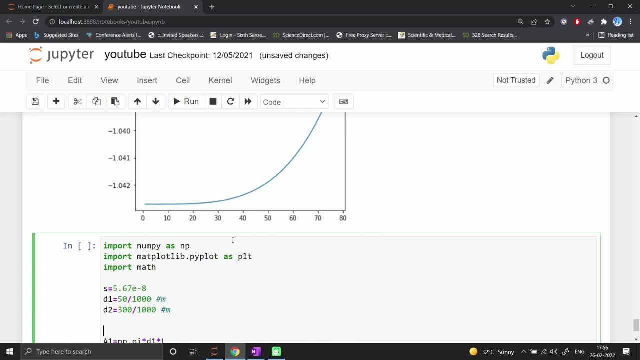 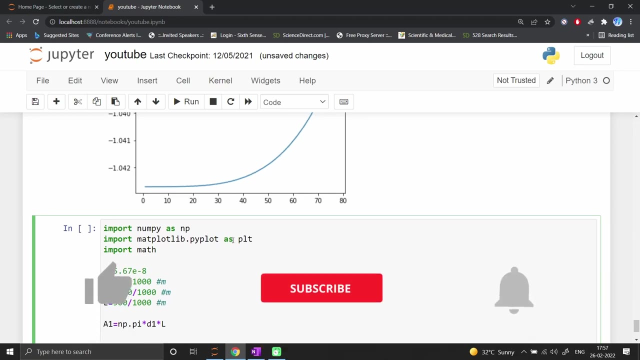 1 multiplied by length, L, so our length is equal to cylinder. length is equal to. L is equal to 500, or 500 divided by 1000 in meter, so it is 500 mm and same a 2. a 2 is equal to numpy and I will change d2, so this is my surface area of cylinder 1. 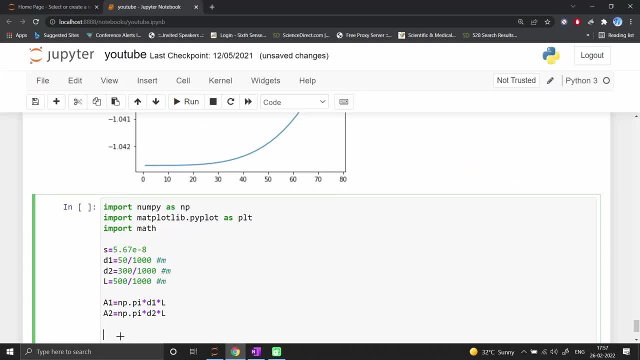 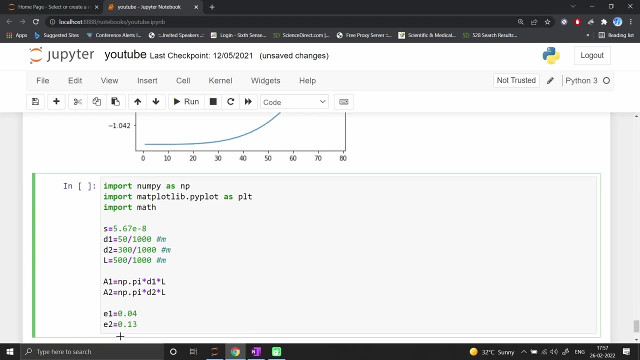 and cylinder 2. now we will define our emissivity. I will say: even is equal to point four, zero four, and e 2 is equal to point three. or I will say: SS property, point 1, 3. now I will define our stufa, miss. Q is equal to Q is equal to s. 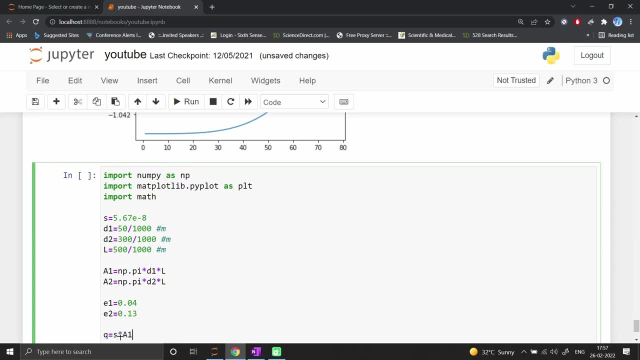 multiplied by a 1, multiplied by, I will define t 1 and t 2. load: t 1 is equal to 4 Kelvin in Kelvin and t 2 is equal to 300 Kelvin. you now I will say T 1 raised to 4 minus t 2. 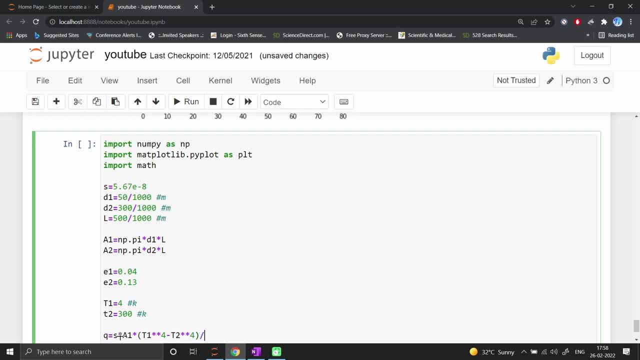 twist to 4, divide by 1 divided by even plus 1 minus e 2 divided by e 2, and this match is a 1 divided by t 3 plus 4 minus T 2, and I will say so, this t 1 is equal to. 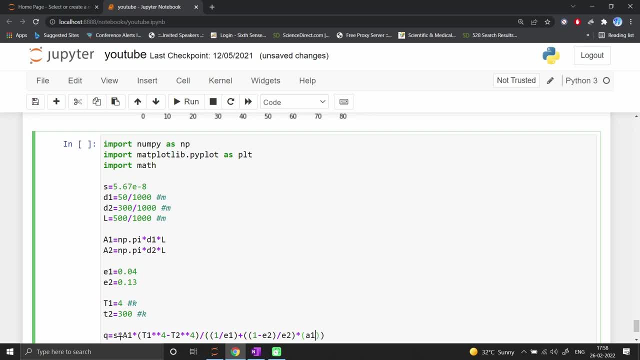 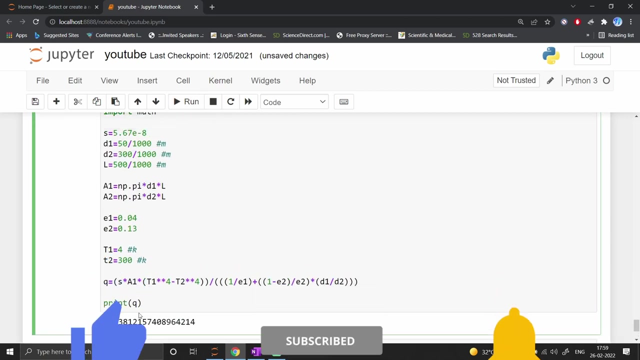 plus minus e 2 divided by e 3, and this multiplication of d1 divided by d2 divided by d2. this is our equation. I'll bracket all this thing so it will not confuse program and I will say: print my cube. this is simple formula. if I run this code, I will say: my heat load is: